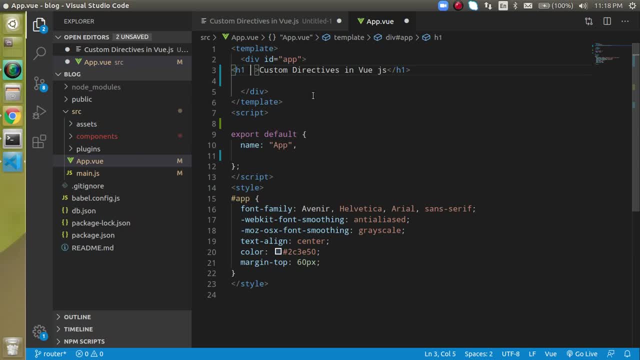 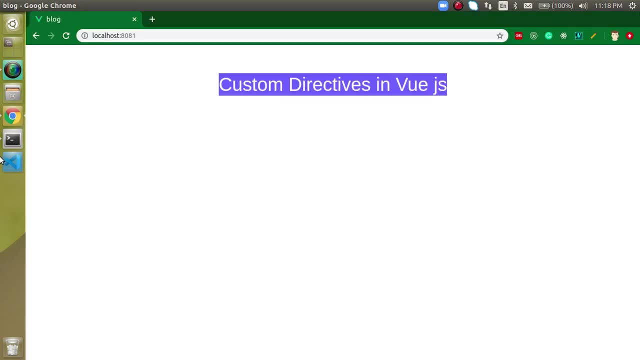 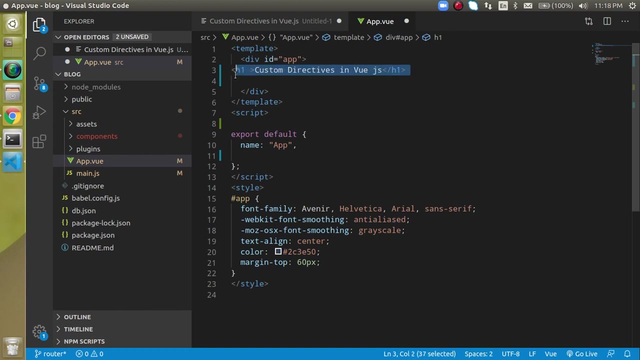 application, when your application is loaded. Alright, so now let's see how we can, what we are just going to make. So here you can see that this is the output of our this tag. Alright, so I'm just going to make a custom directive that will just make it small, medium and large with the help of value, Right? So now let's see. So for that, let's say I just want to make the name of this custom directive is: 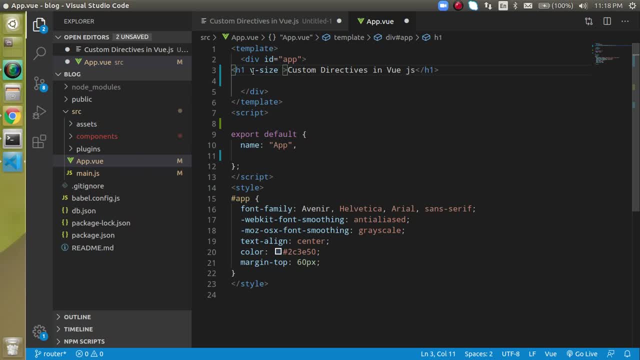 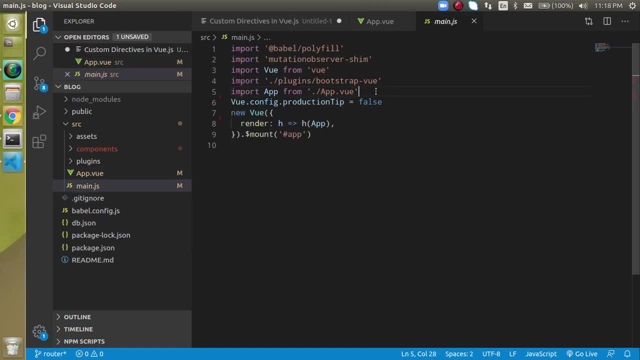 size. So I have to define it with the V hyphen size Right. So now to use it or to define it, just go inside the mainjs and just simply use here view dot directive, And it have the two parameters. One is your. 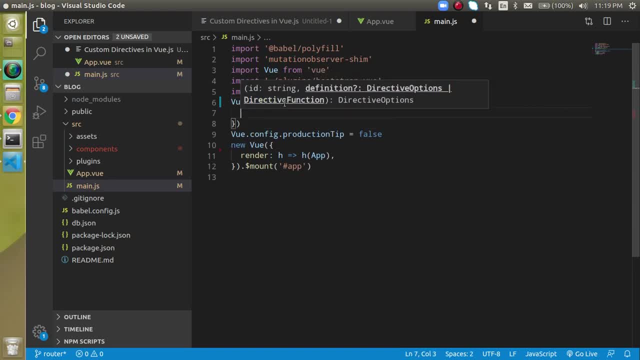 active name, which is size. And second, one is basically a object, Right, And in this object we have a bind function And it has a three value. one is here, that is element, Second is binding and third one is V, node Right. So for a moment I will just only use 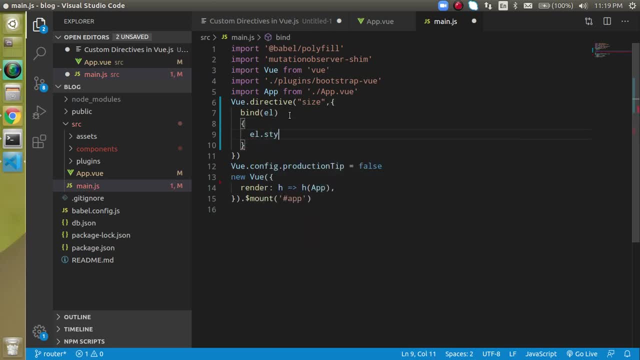 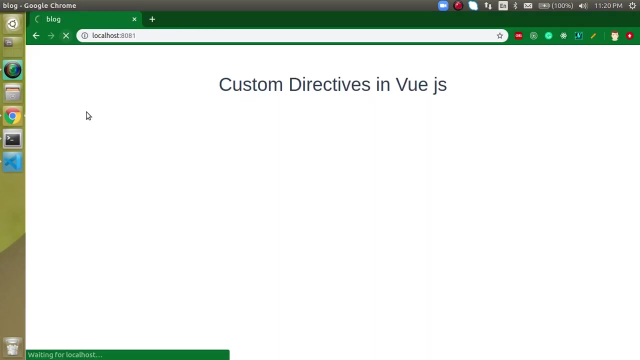 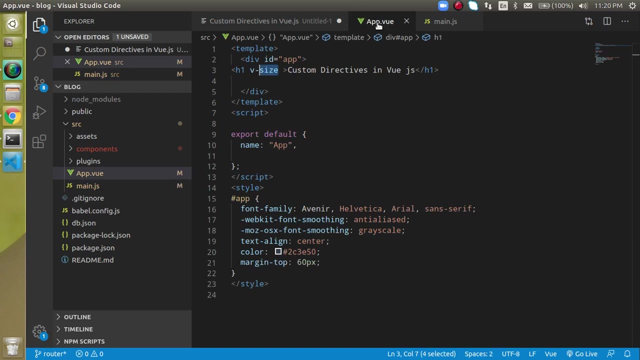 EL. So just we can use here EL dot, Style dot. font size. font size can be like 100 pixel and it should be inside the courts. So now let's see Make a refresh on it And now you can see that the size of this text is change. Alright, so this is. you can say that this is our basic of custom directive. So if you just want to make some copy, so 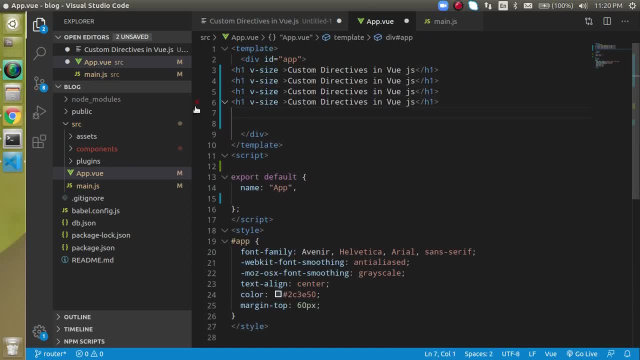 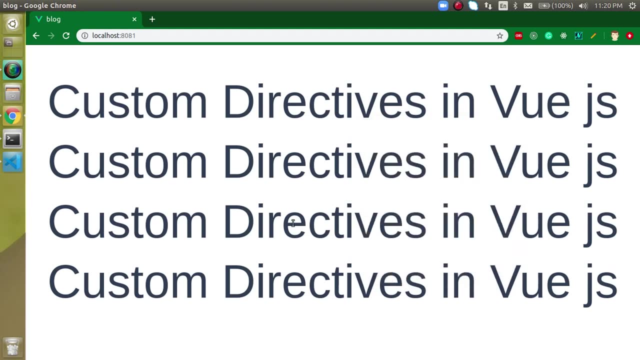 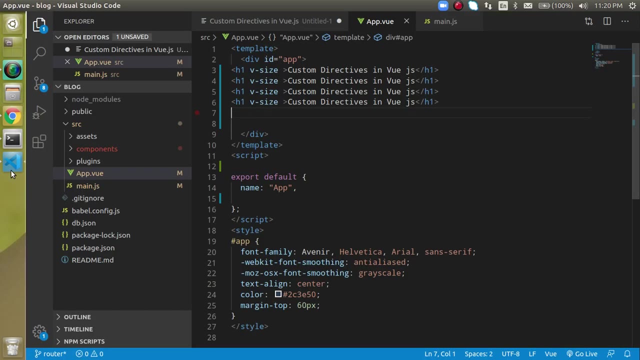 copy uties things or you just want to make in the any another component. you can just simply use it like this: right, everywhere the font size is applied here. you can see that in the inspect element part also, size is 100 pixel for everyone. all right, but this is the default value. 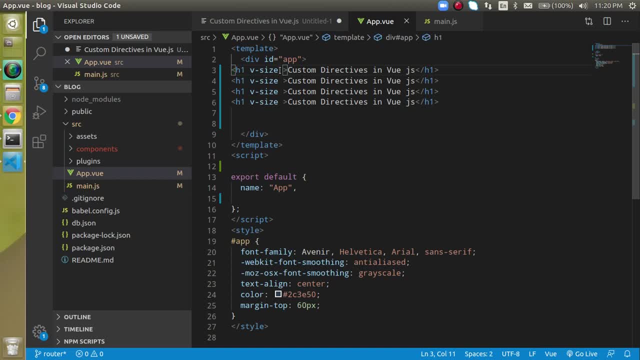 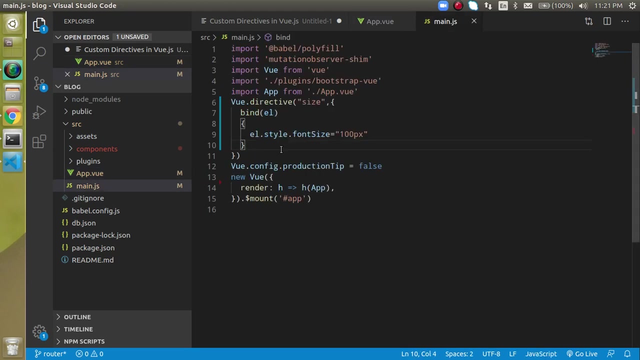 just i want to make some, uh, defined value. so just i want to make it small, like this, all right. or i i just want to make it medium and large, and all right. so for a moment i'm just going to remove it, and now let's see how we can just use this value here. so here i can just use. 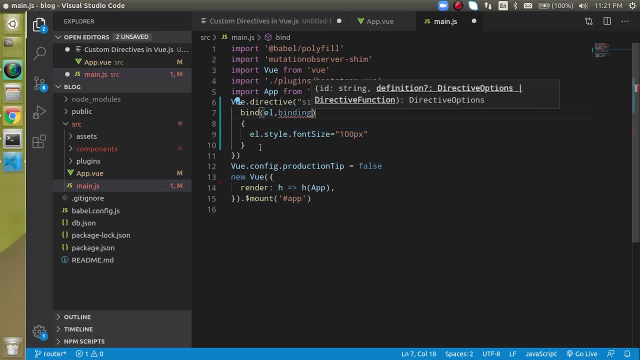 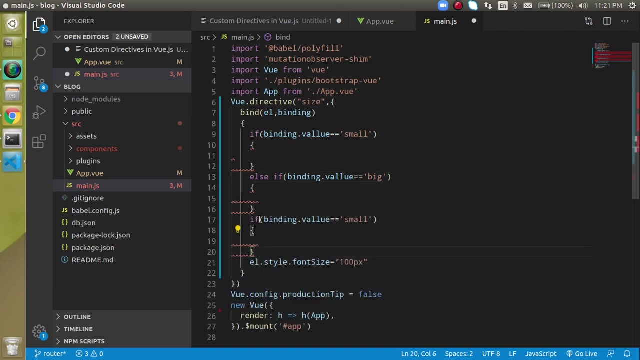 comma binding right and just use here: if binding dot value equal, equal small right, then we have to run a condition. after that we can also run else if, if the value is big and at the last we can also run a else condition. just we don't need it right. and 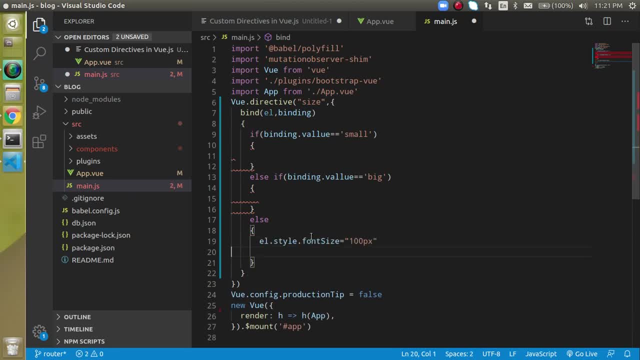 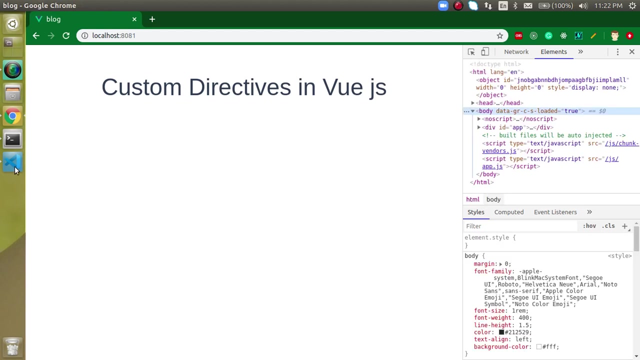 just put this here here. all right. so if we have a small size, then font size can be a 20 pixel, perfect. if we have a big size, then 150, and if have this normal size, then we can have a 50 pixel, all right. so now we have a. what is the value of? 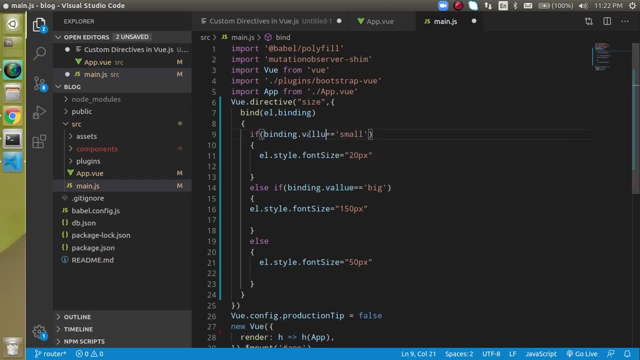 okay, i just have to use a value here. this is my mistake, let me correct it. yep, so now you can see that the small size is small, because this condition is matching here. here you can see that. all right, so i just want to make the two more condition. 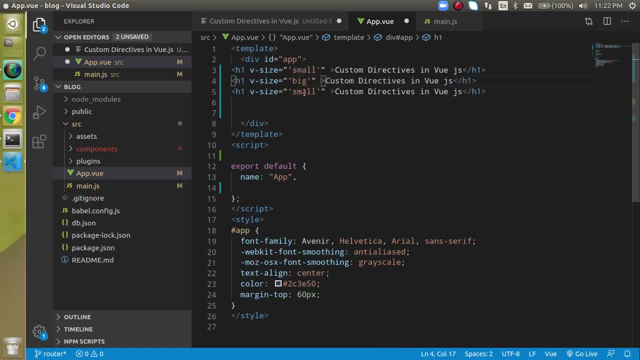 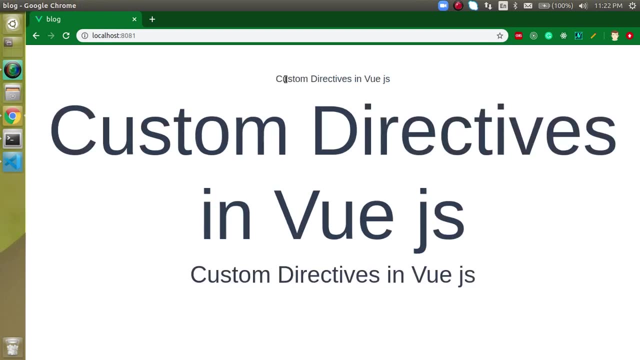 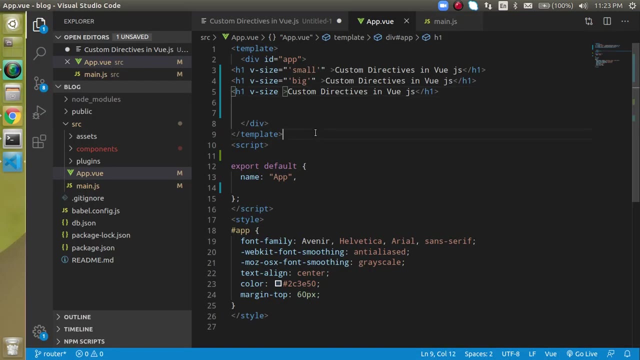 so now i just want to make a big, and here i can i just remove to all values. then what is going on? so here you can see that first of all the small case is made match, then big and then the normal case. all right, so this is the way that how we can just change the style with custom directives and we can pass the value. 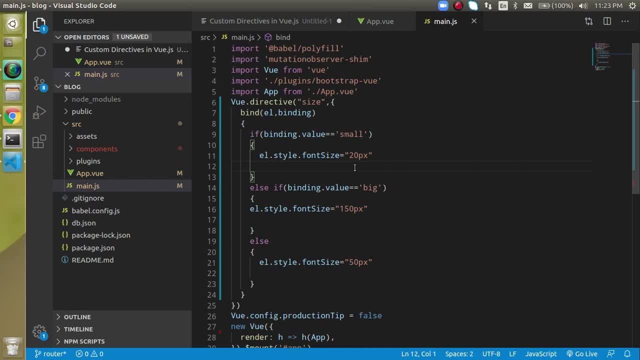 also, if you still have any kind of confusion, you can ask me in the comment box. don't forget to subscribe my channel and like this video. bye, bye, take care.